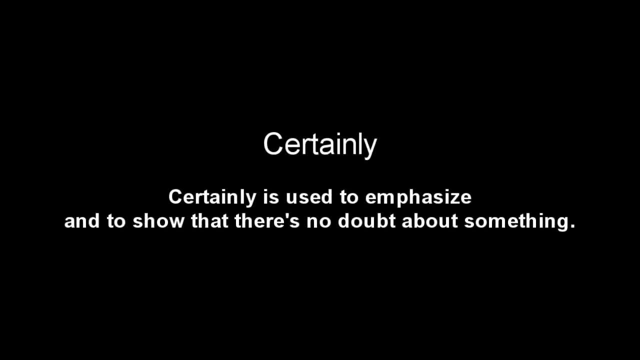 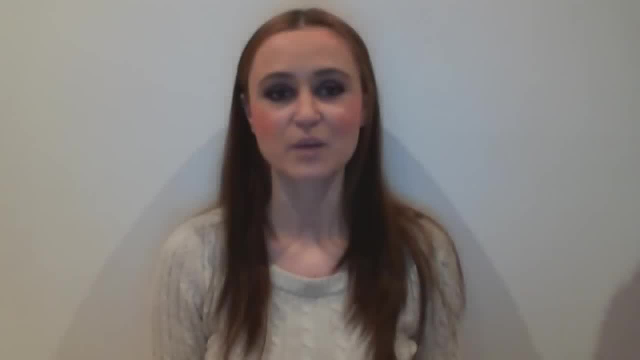 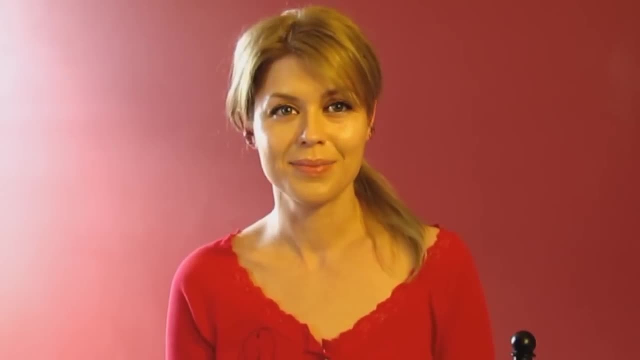 Certainly is used to emphasize and to show confidence, To show that there's no doubt about something. Paula, I wrote you a blog yesterday. You're such a great writer. Thanks, I'm glad you liked it. Have you always wanted to become a writer? 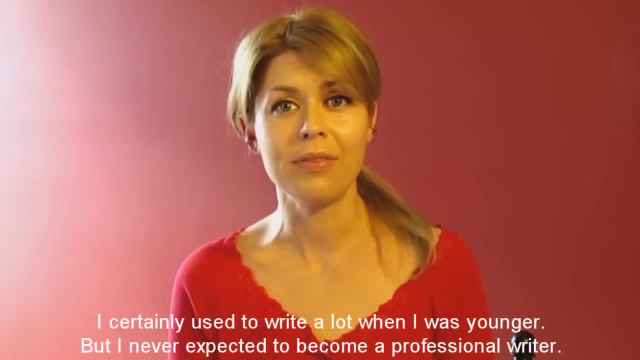 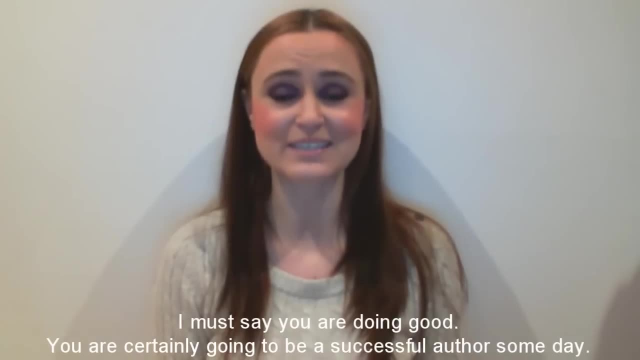 I certainly used to write a lot when I was younger, but I never expected to become a professional writer. I must say, you're doing good. You're certainly going to be a successful author someday. Well, there's certainly a long way to go. 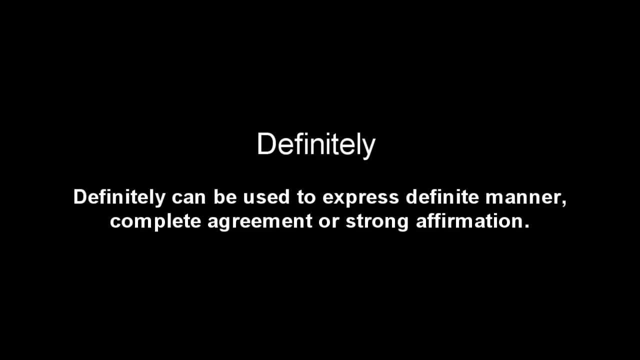 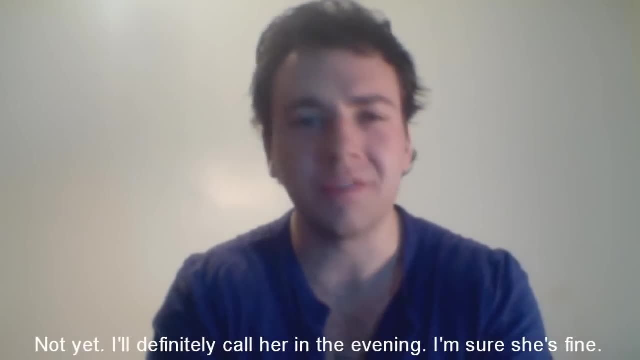 Definitely can be used to express definite manner, complete agreement or strong affirmation. Mark, did you call your mother? Not yet. I'll definitely call her in the evening. I'm sure she's fine. I'll most definitely not accept any excuse this time. I want you to call her right now. 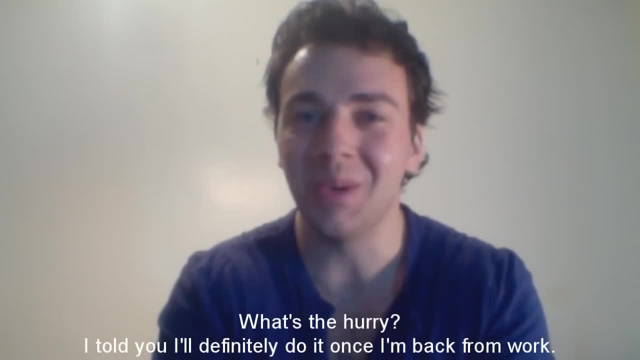 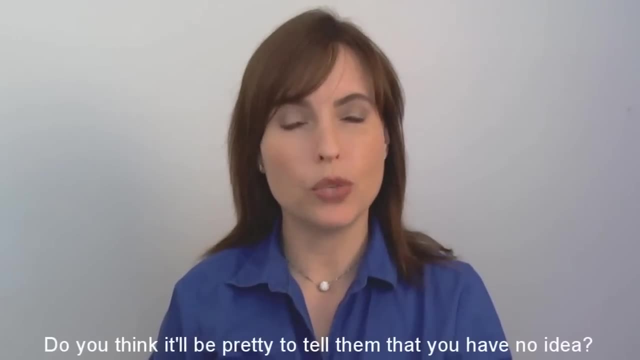 What's the hurry? I told you I'll definitely do it once I'm back from work. Your relatives are coming over. They'll definitely ask you for some news about her. Do you think it'll be pretty to tell them that you have no idea? 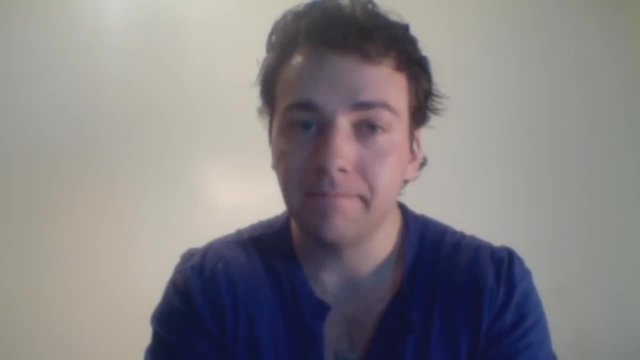 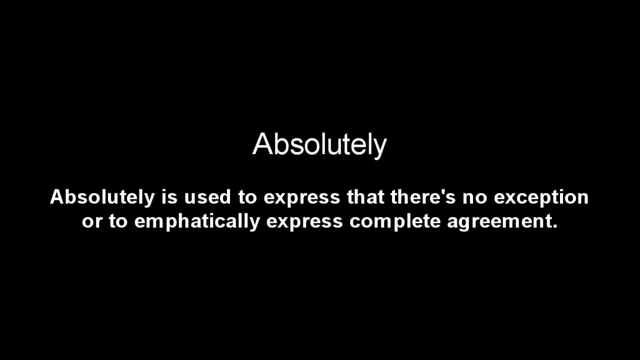 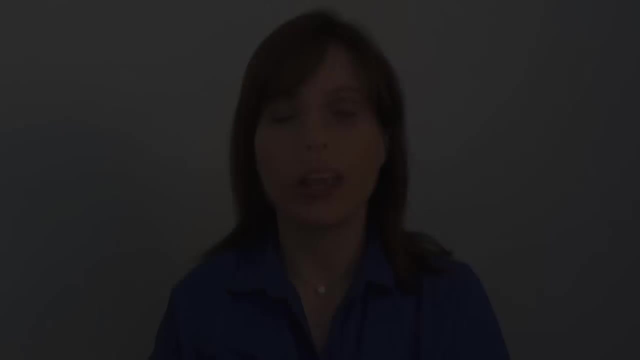 No, definitely not. I'll call her now. Absolutely is used to express that there's no exception, or to empathetically express complete agreement. I absolutely want to do this. Mark, Do you have any idea what you're saying? Why do you want to resign? 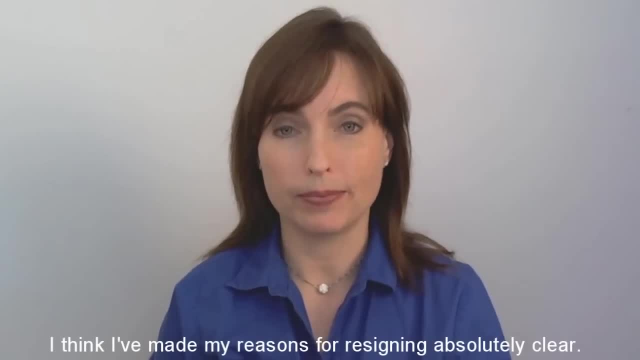 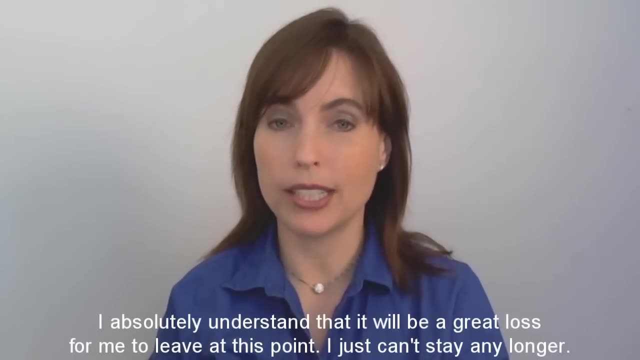 I think I've made my reasons for resigning absolutely clear. I understand your reasons, Mary, but we've been considering you for a promotion. I absolutely understand that it will be a great loss for me to leave at this point. I just can't stay any longer.